They're created by the release of stress- See Giant's Causeway, formed at a volcanic fissure where lava spilled onto the Earth's surface, And, in general, as lava cools, its surface layer shrinks and solidifies, which puts an. 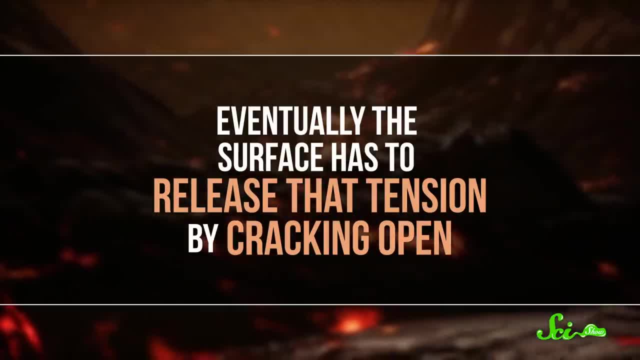 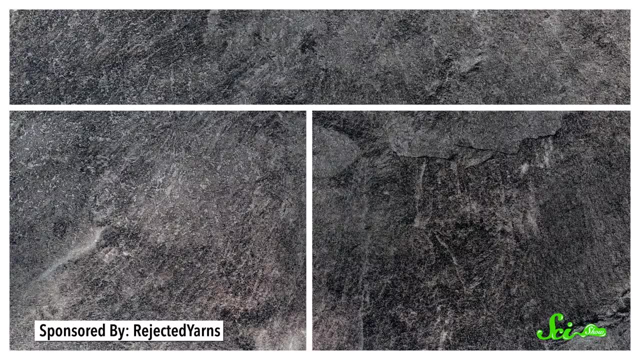 increasing amount of tension on the rock. Eventually the surface has to release that tension by cracking open. Now, at first the cracks form at random And they tend to criss-cross, because perpendicular lines can release the most energy from the rock. But then, as the lava cools from the top down, each lower layer of lava cracks also. 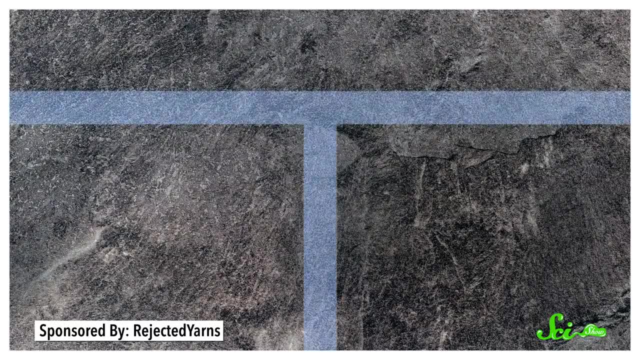 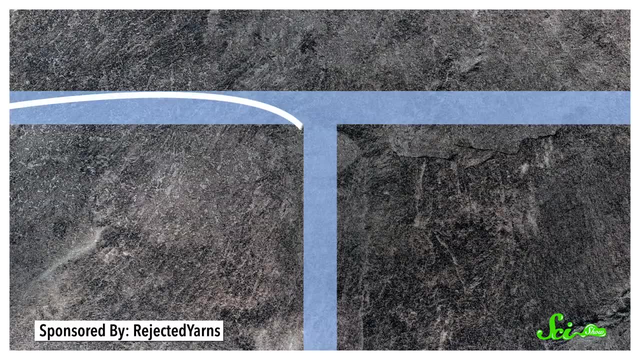 And that's what we're looking for. Usually, the new cracks form right below the existing ones, because the rock is already a little bit weaker there. But instead of forming a T-shape again, the new cracks literally cut corners to release more energy. 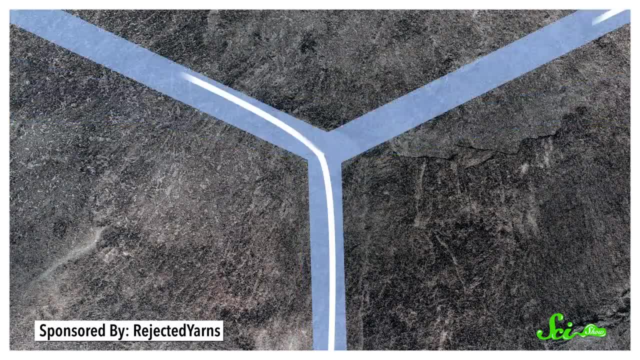 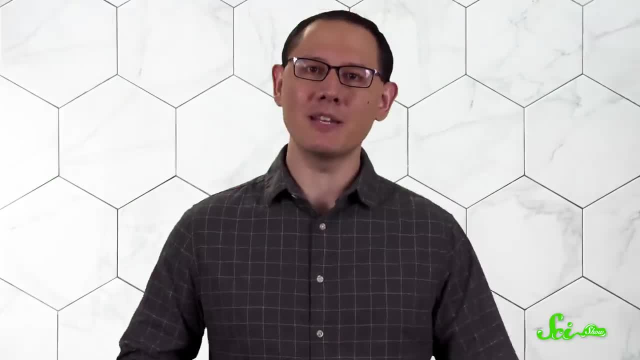 So as the crack gets deeper the T-shape gets more rounded, until eventually it looks like a Y with equal angles. And if you have a bunch of Y-shaped intersections next to each other you end up with hexagons. So at Giant's Causeway, cracks formed columns in the hardened lava. 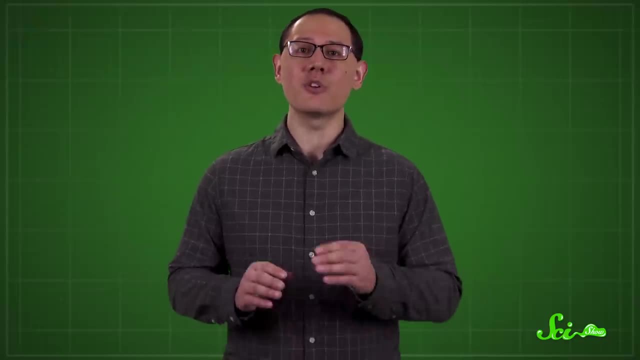 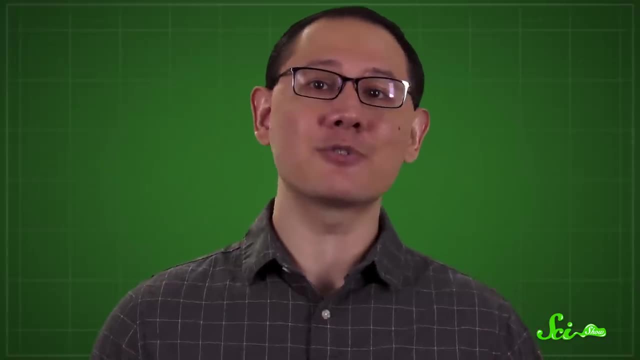 And as that rock erupted, cracks formed columns in the hardened lava. But when the rock erupted down, it exposed those Y-shaped columns, Meaning that in the end, this grandiose natural structure was likely all the result of some pretty basic physics. 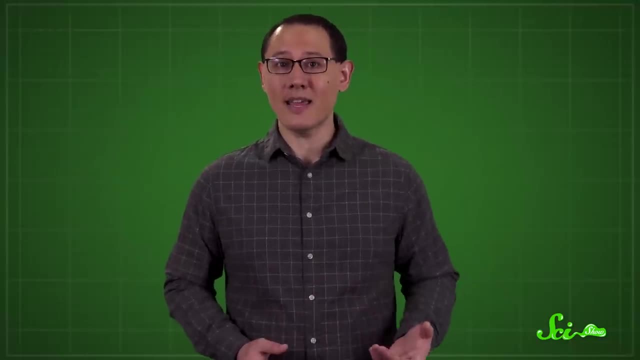 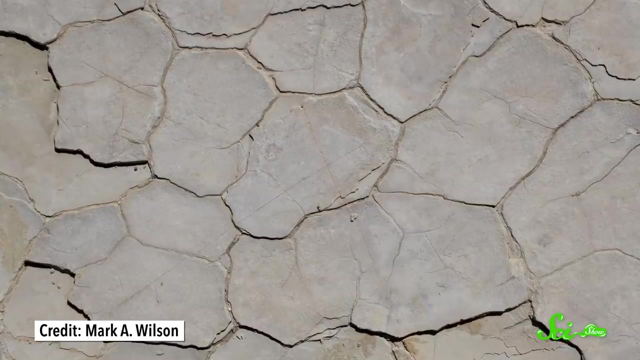 And in other natural places where we see hexagons like the cracks in glaze or dried mud. scientists think something similar is happening. It's just that in these cases, instead of growing deeper, the original cracks are closing up and then reforming during cycles of heating and cooling, or wetting and drying. 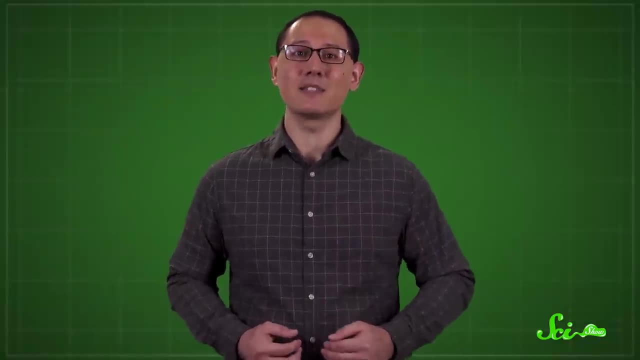 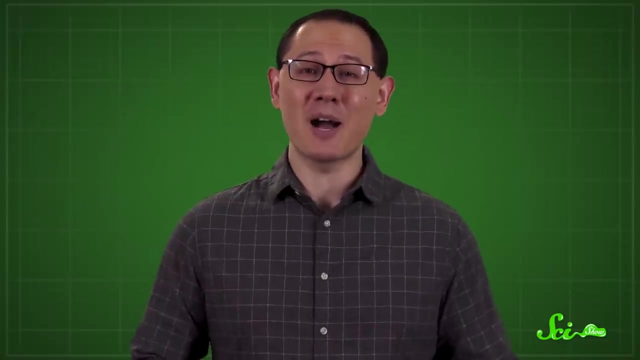 And each time they split open again, they tend to crack along the same lines. but just Just like the cracks in lava, they will also cut corners until the T-shapes have evolved into Ys. So, even though a glazed pot and a dry lakebed don't have a lot in common- simple physics. 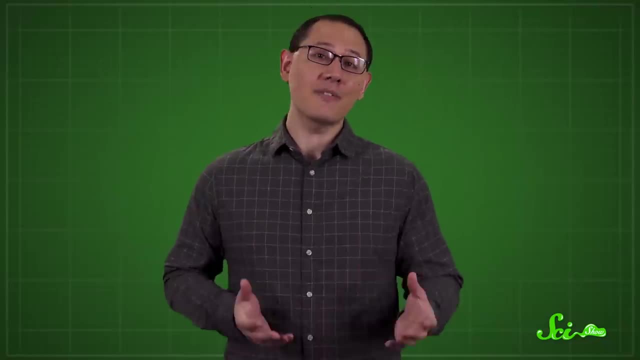 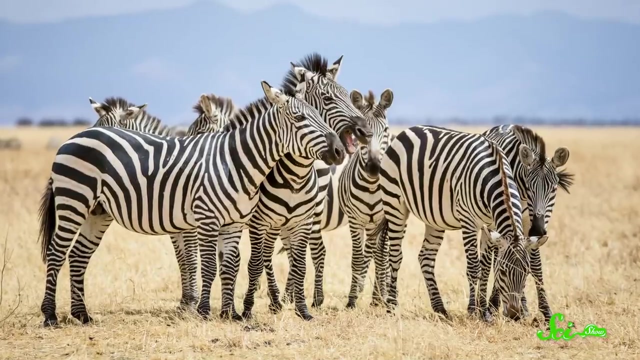 may explain the strangely similar patterns on both of them. Now, if you haven't noticed the hexagons in nature before, one emergent pattern you've almost certainly noticed is stripes. Take zebras, for instance. They might be one of the most famously striped creatures, but the pattern is far from unique. 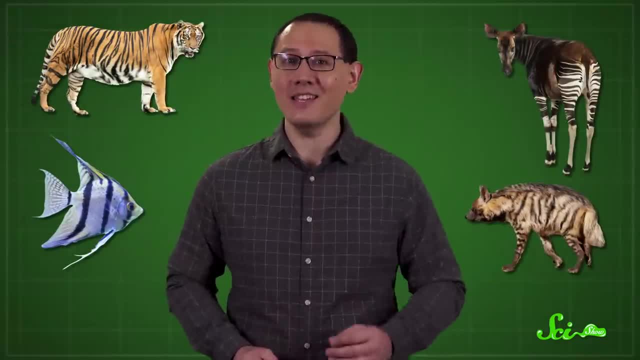 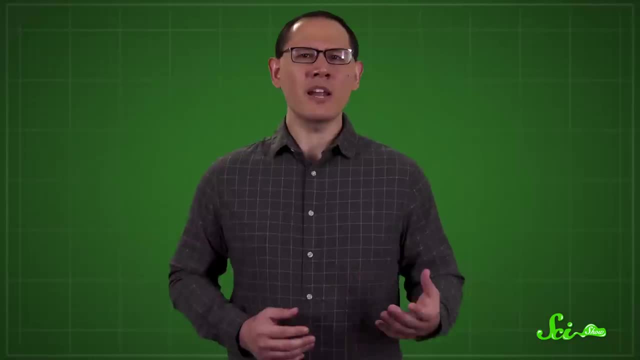 to them. Things like tigers, okapi, angelfish and certain hyenas all wear stripes too, and none of them are closely related in terms of evolution, But they actually might have something in common. One idea that scientists have investigated for years is that zebra stripes form through 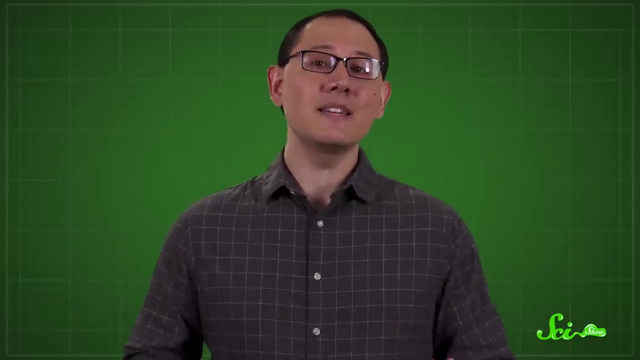 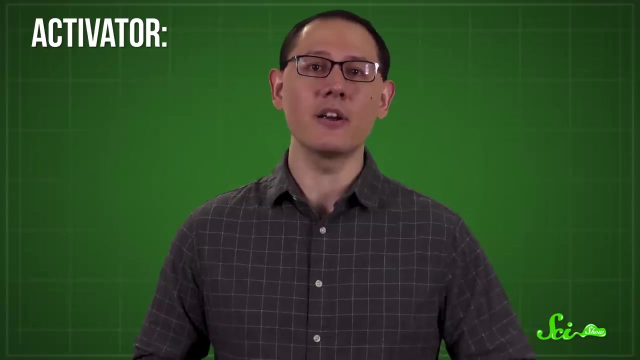 a chemical process called a reaction-diffusion system. The idea is that as a zebra's body grows, at little points throughout, its skin cells start to make a protein or chemical called an activator. that does a few things. First, it signals to skin cells around it to start producing pigment, turning that patch. 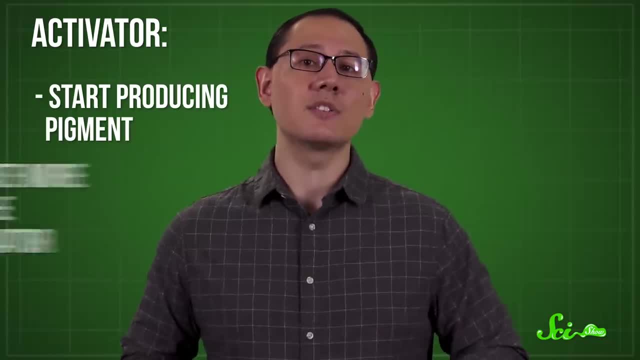 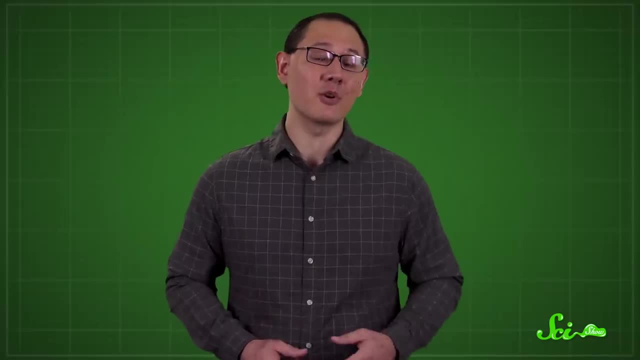 of skin a source of oxygen. Second, it tells those cells to create more of the activator. So since it essentially self-multiplies, the signal from the activator will spread and get stronger over time. This means that if left alone, even a little blip of this chemical on the zebra's nose 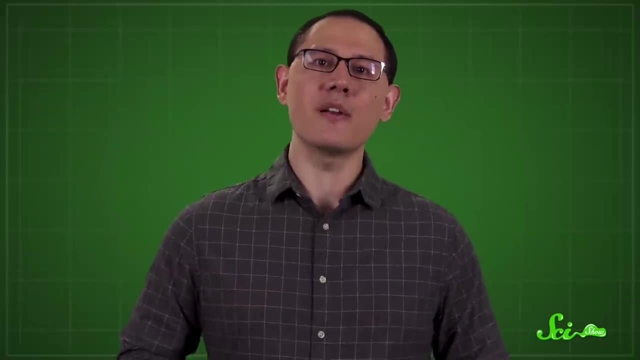 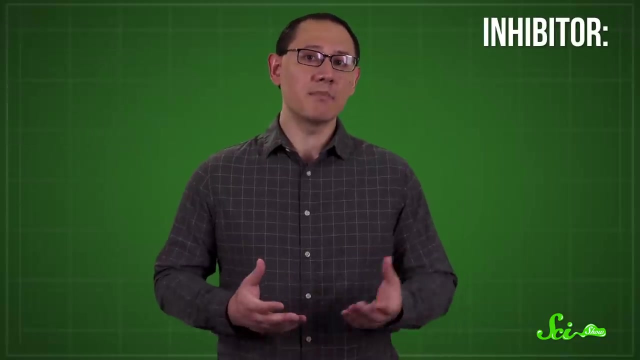 would turn the whole animal black. But it doesn't just go on forever, because the activator also does one more thing: It tells the cells to produce something called an inhibitor, And an inhibitor is some chemical or protein that puts a stop to the self-multiplying behavior. 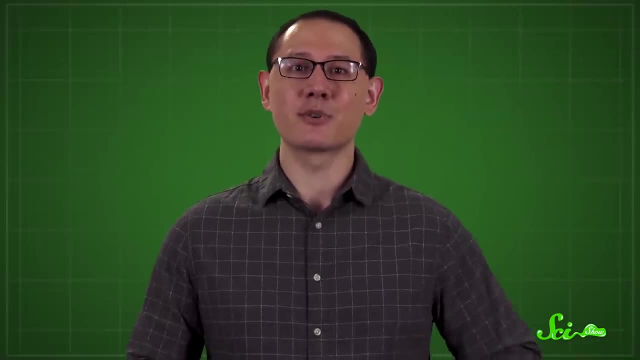 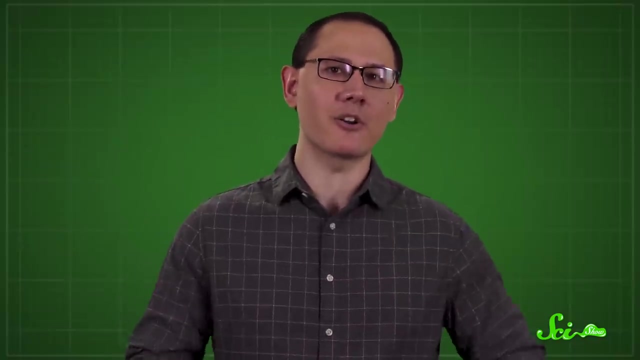 and breaks the cycle. So the activator is sending mixed messages. It's creating one chemical that says turn black and make more of me, and another just behind it that says ignore that order For the first few cells. that second message may come a little too late. 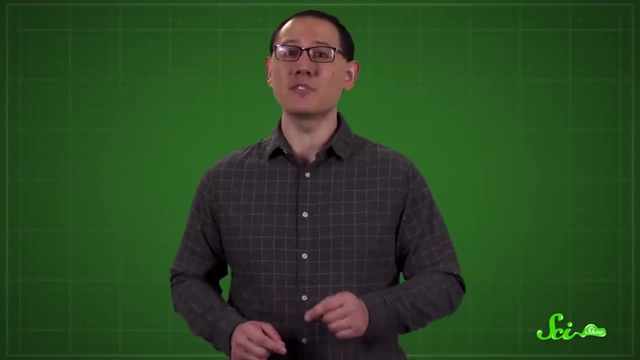 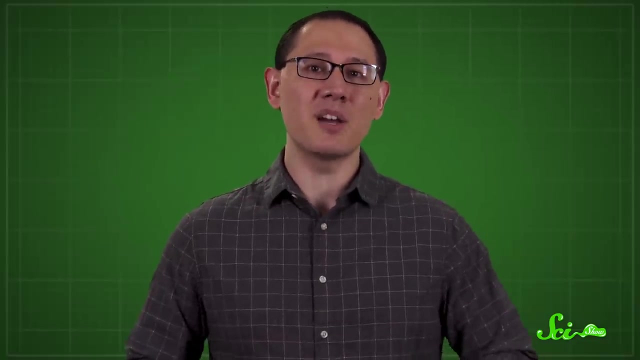 The cells are already destined to become black. But the inhibitor actually moves a little bit faster than the activator, In other words, it diffuses faster. The reason may vary from one inhibitor to another, but, for example, maybe it's a little. 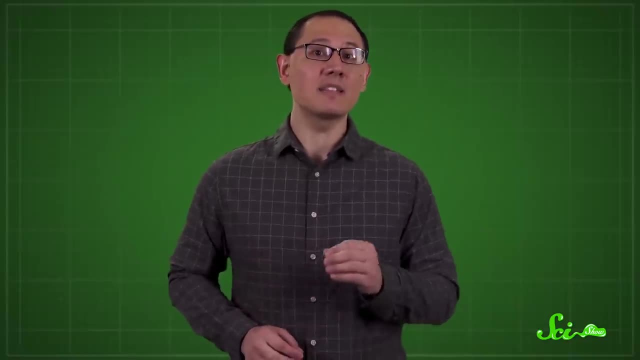 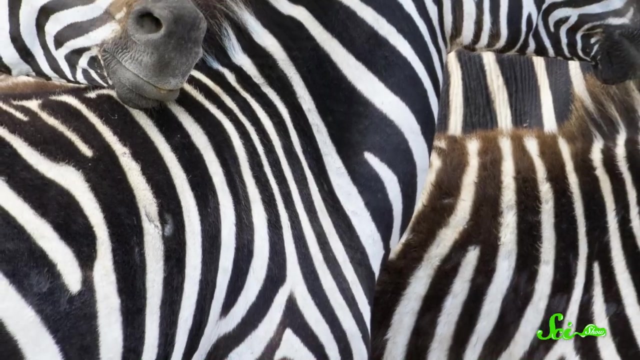 smaller. But either way, eventually the inhibitor catches up. Getting the inhibitor out of the way is a good thing. It's getting its message across in time to stop the activator. So it ends the stripe and leaves a patch of white. And if you have this scenario play out over and over across the zebra's body, you'll. 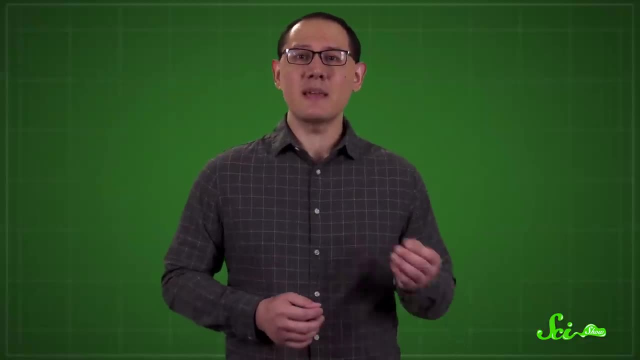 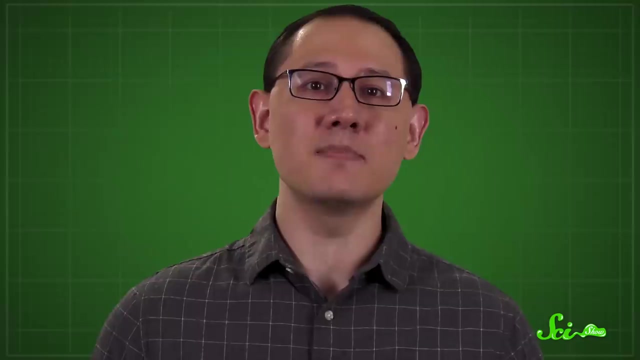 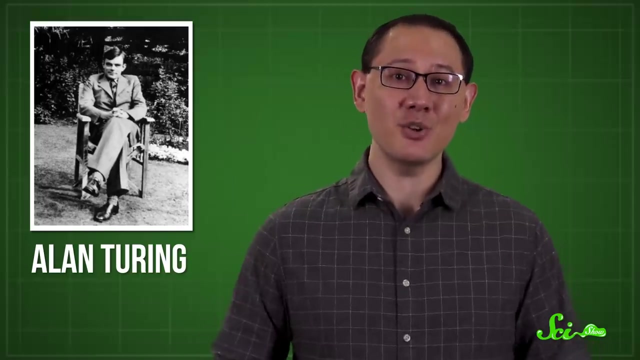 end up with those famous stripes, And with a slightly different setup, the same mechanism can also create spotted patterns, spirals or maze-like ones too. The thing is, for a long time this mechanism was purely hypothetical. It was proposed by the British mathematician Alan Turing, who put out a paper in 1952 outlining 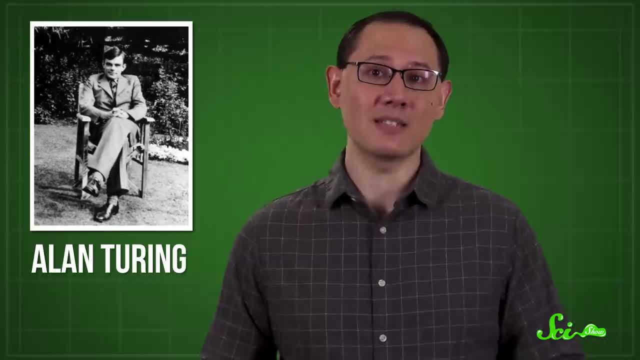 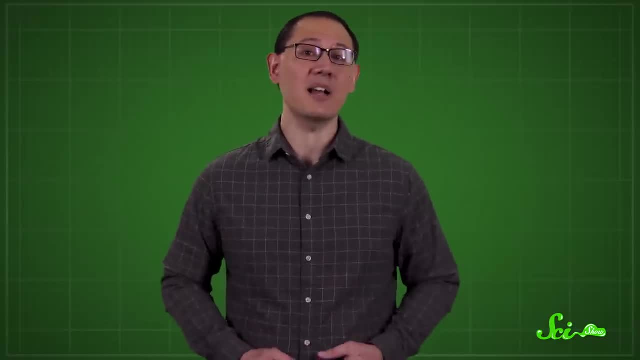 how animal patterns like stripes or spots could emerge through this mechanism, And chemists had noticed similar oscillating patterns in chemical reactions since 1910.. So it did seem possible, But for decades no one could prove that chemicals like this were creating these so-called Turing. 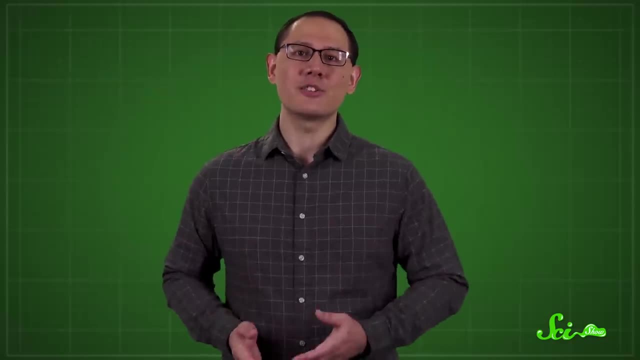 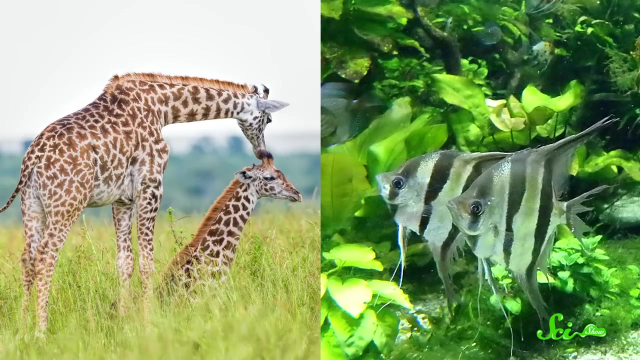 patterns in animals. But today scientists have done a lot more research and they've spotted what look like Turing patterns all over nature: in angelfish stripes, giraffe spots and even the arrangement of feathers and hair follicles in the skin. 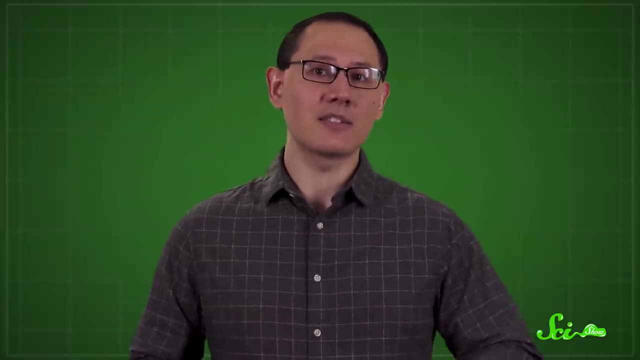 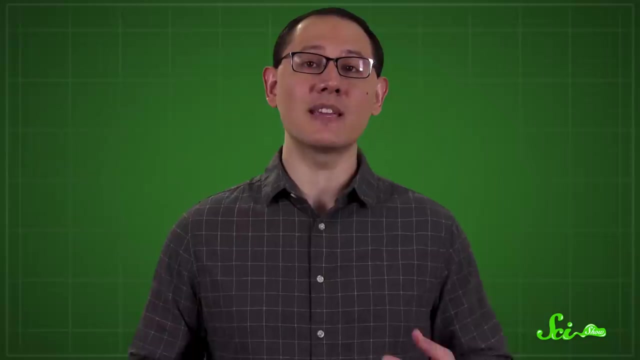 They've even taken things one step further And in some examples, like the stripy pattern of ridges inside the mouths of mice, they've been able to nail down the exact identity of the proteins working as activators and inhibitors. So all over the biological world there are patterns that appear to be related to this. 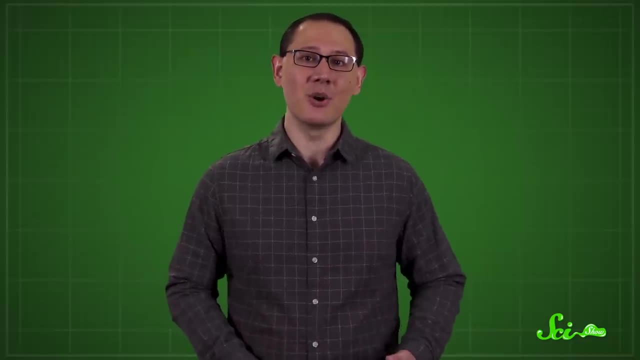 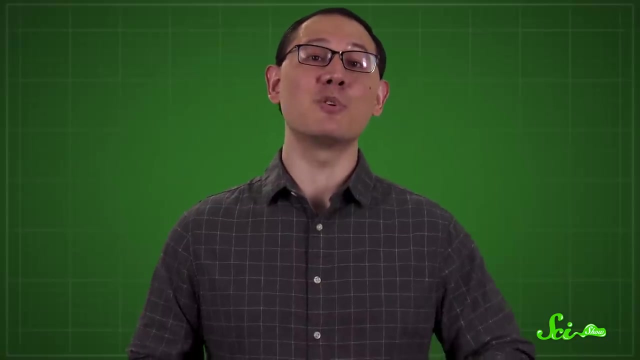 simple mathematical idea that Turing proposed in 1952, including some less obvious ones, Like in 2012,. scientists even suggested that Turing patterns might be responsible for fingers. Their study found that in mouse embryos, fingers develop as the most important part of the 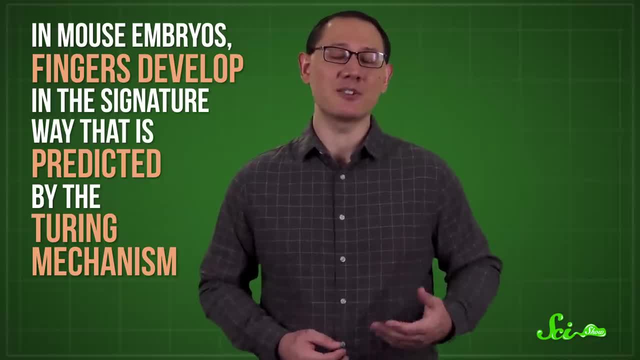 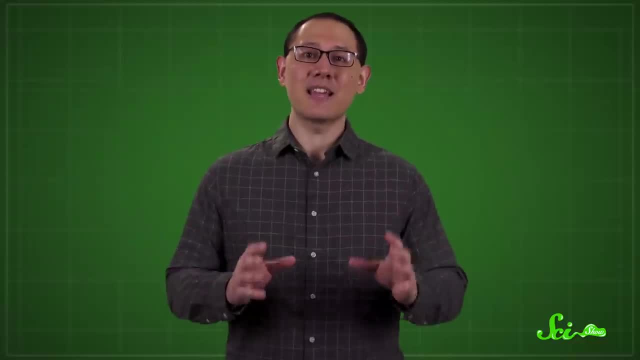 body in the signature way that is predicted by the Turing mechanism. If they're right, that means we could think of fingers as… maybe just really weird stripes, But in any case, scientists are still exploring Turing's hypothesis, and the mechanism he described can even be applied to patterns that aren't biological. 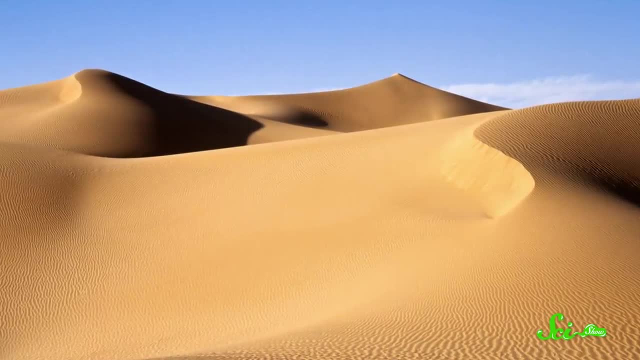 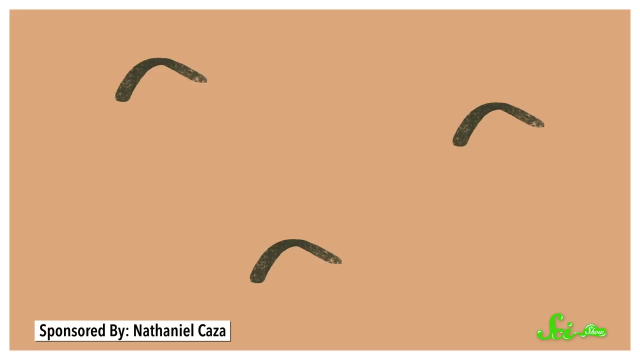 For instance, sand dunes are purely physical patterns, but you can think of them as following the same principles of activators and inhibitors. See: sand dunes form on flat, windy land that's full of small imperfections, like a boulder or a little ridge. 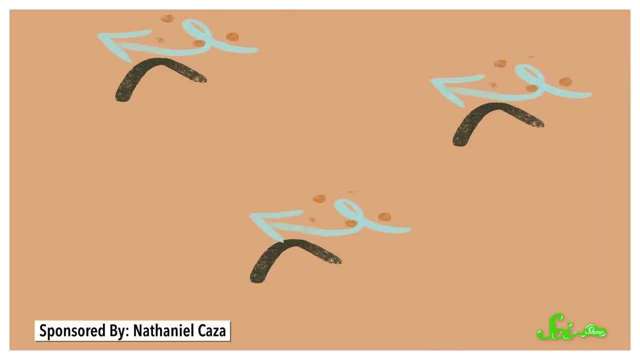 As the wind blows it meets those small imperfections which break up the air current. As soon as the current is gone, any dust or sand the wind was carrying falls and builds up on the downwind side of the imperfection And over time this little pile grows and as it gets bigger. 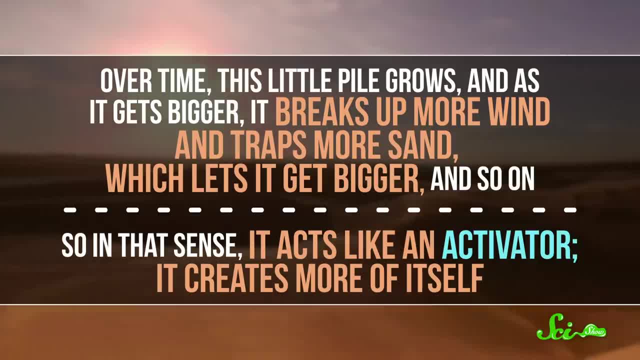 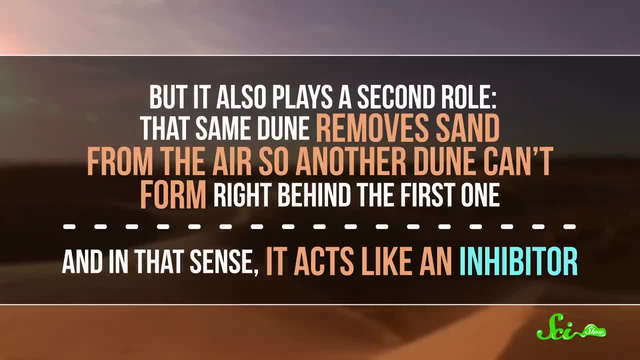 it breaks up more wind and traps more sand, which lets it get bigger, and so on. So in that sense it acts like an activator. It creates more of itself. But it also plays a second role. That same dune removes sand from the air. 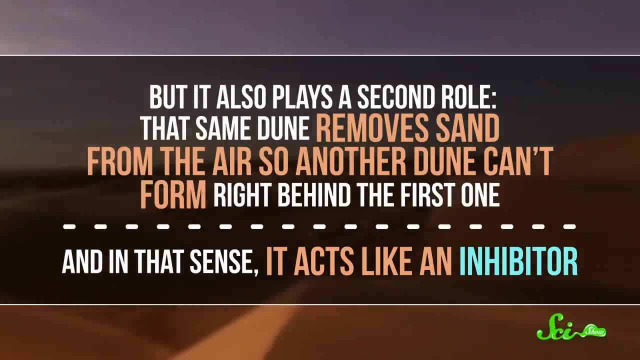 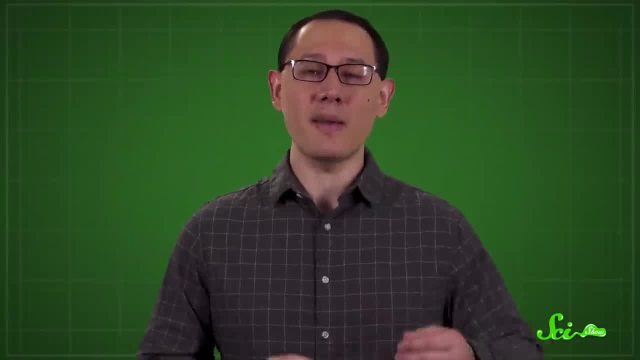 so another dune can't… form right behind the first one, And in that sense it acts like an inhibitor. So in a way, the naturally spaced out ridges we see in dunes arise from the same principle. that may create zebra stripes.